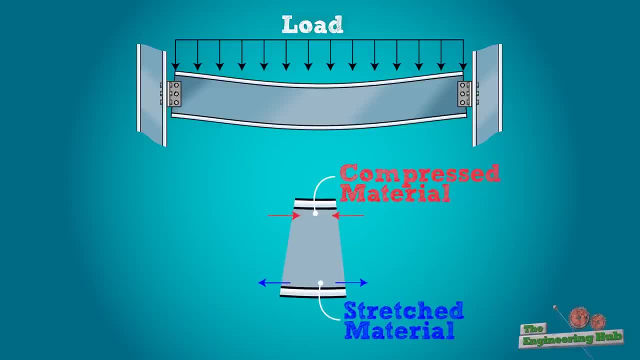 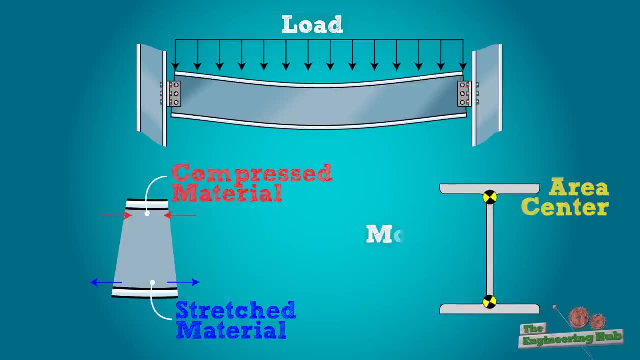 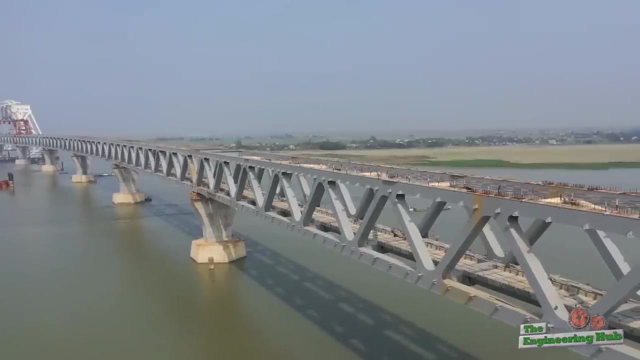 to the end supports. The further apart these forces are, the higher the bending capacity of the beam is. Hence why the wide flange beams have most of their cross-sectional area offset to the top and bottom of the beam. The truss takes this concept to the next level. If you think about it, the truss is. 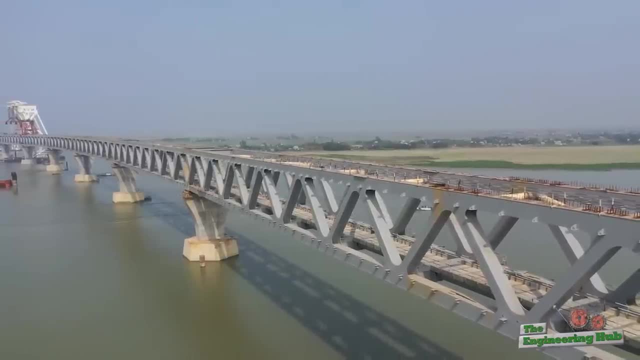 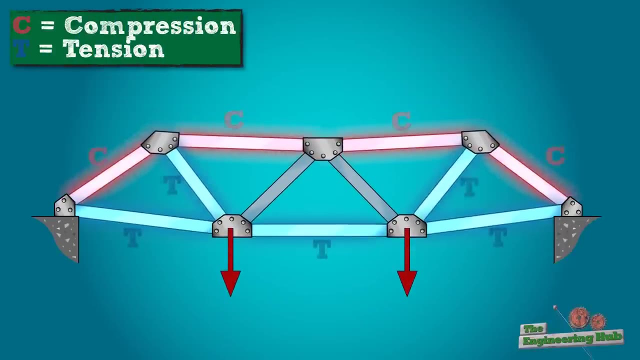 basically a beam where the top and bottom flanges are structural members of their own. The beauty of the truss is that all of its members are only subjected to axial loads, which makes the whole structure efficient and also incredibly stiff. This may not be. 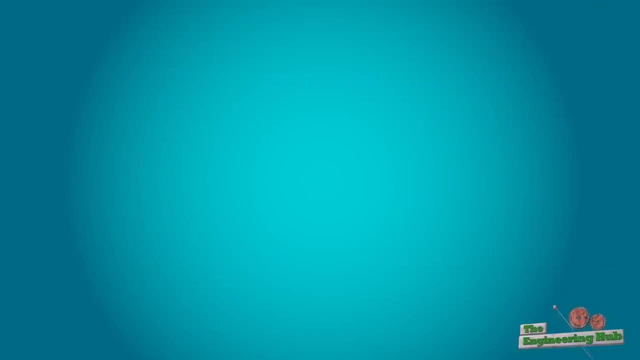 obvious. so let's have a deeper look. But just to be clear, stiffness in engineering terms means the amount of load a structure can take per unit deformation. Or another way to think about it is what load causes the structure to deform by one millimeter. 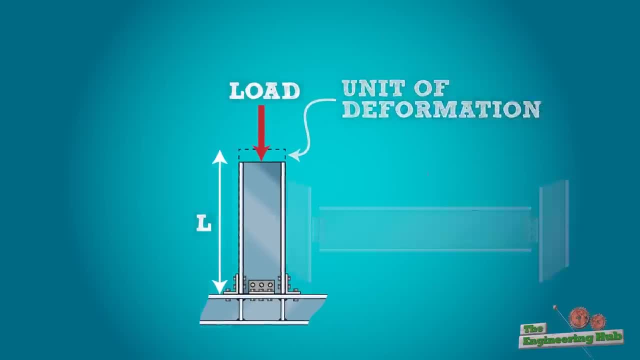 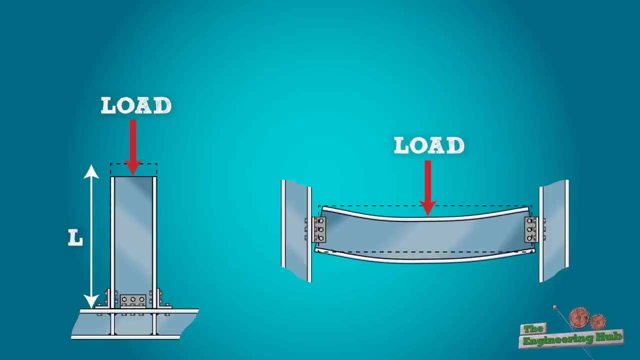 or one inch or whatever unit you prefer. Intuitively, you know that it is much easier to deform a member by bending it rather than compressing it. So it follows that bending members, such as beams, exhibit low stiffness for longer spans. This is because the stiffness of a 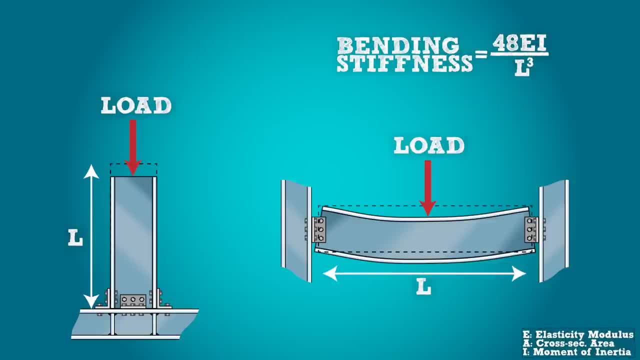 simple beam is scaled with the cube of the length of the span. This means that doubling the length makes the beam more flexible and therefore less flexible. This means that the beam eight times more flexible. If you have worked with long beams, you have probably noticed how. 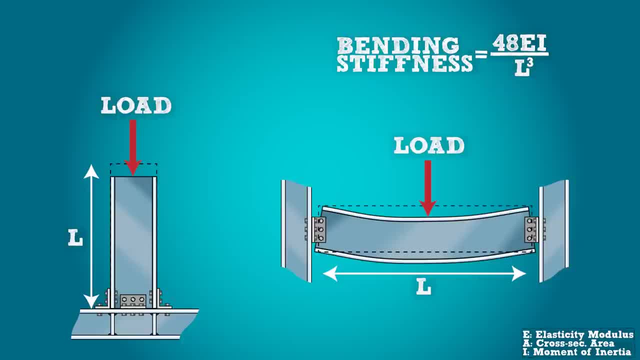 wobbly. they are compared to shorter beams of the same cross section. Now, trusses do not have bending members, so this formula does not directly apply. Trusses are arranged in such a way that all of its members are loaded axially. The stiffness of axially loaded members scales linearly with the 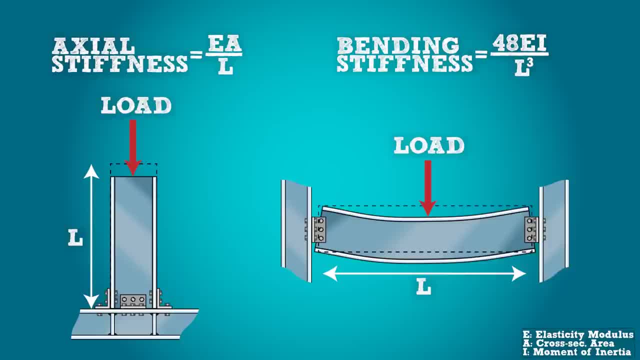 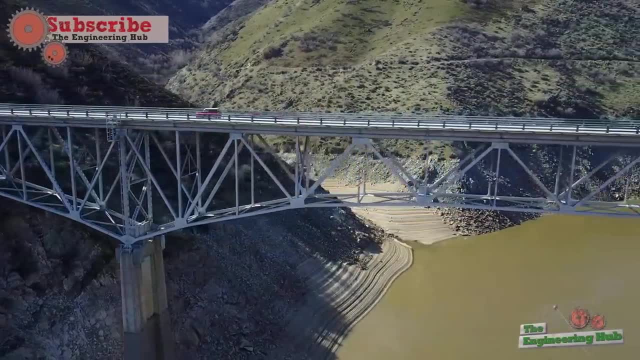 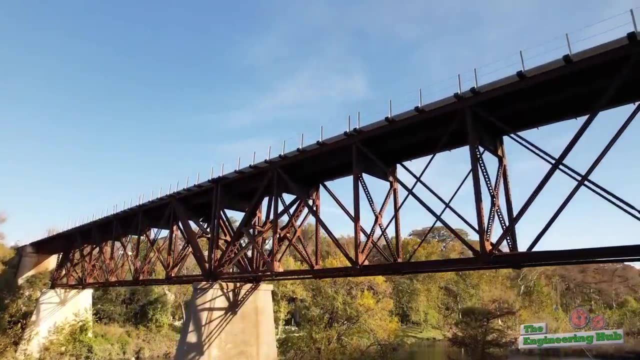 length. So axially loaded assemblies are naturally more suitable for longer spanning structures such as bridges. However, it takes a little bit of thinking to arrange such assemblies of elements in a way that all of the members are axially loaded, yet they span a longer distance. One way. 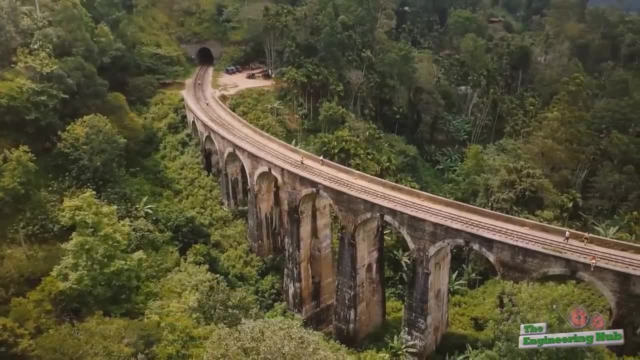 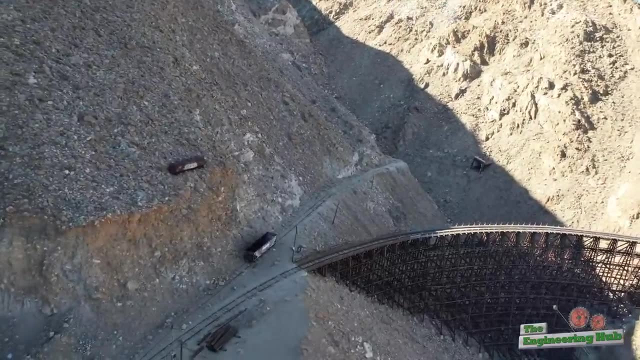 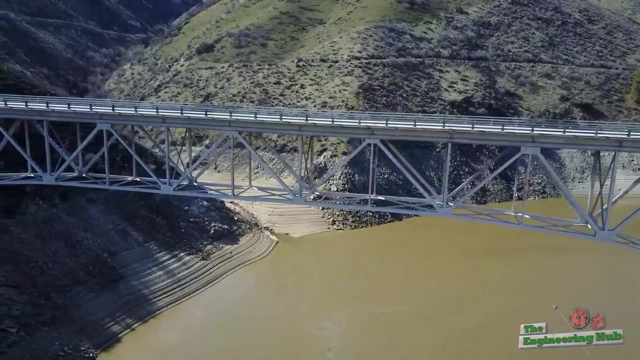 to achieve this is to construct an arch or a trussle bridge, as our ancestors did. Still, these bridges require frequent piers that are not always possible, especially not in deep waters. The truss is an alternative structure that doesn't require regular supports and yet uses the axial stiffness. 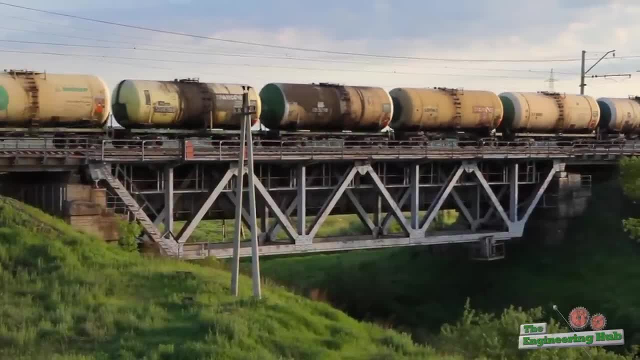 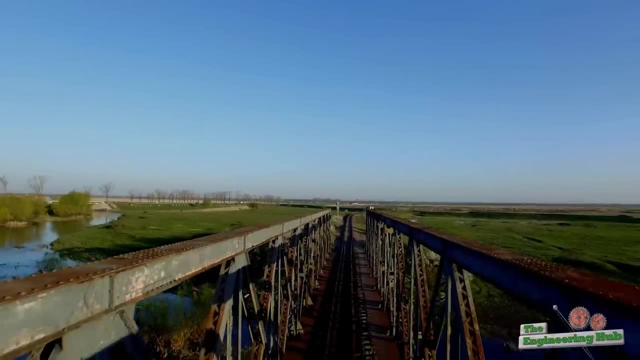 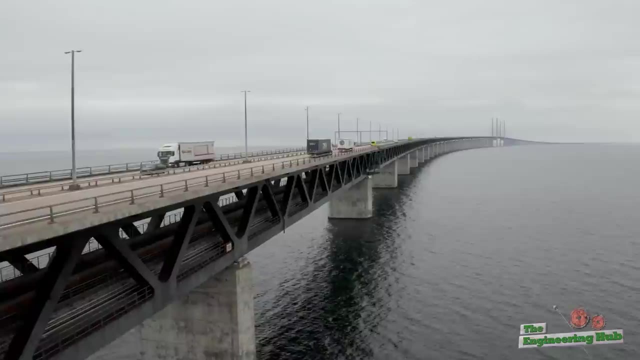 of its members. In fact, the high stiffness of the truss is why it is often used for railway bridges. Railways have very strict deflection requirements because an excessive deformation of the bridge and rail would lead to a derailment of the train. For that reason, even today, bridges that serve as 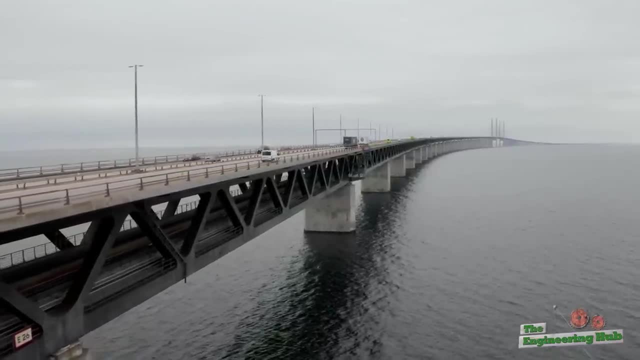 a rail connection utilize some sort of a truss structure within them. Suspension bridges, due to their high stiffness of the truss, could be used as ayu travel variety and then used as a suspension bridges would be used as a waiting place for a temporary образом For the rail to be used for a 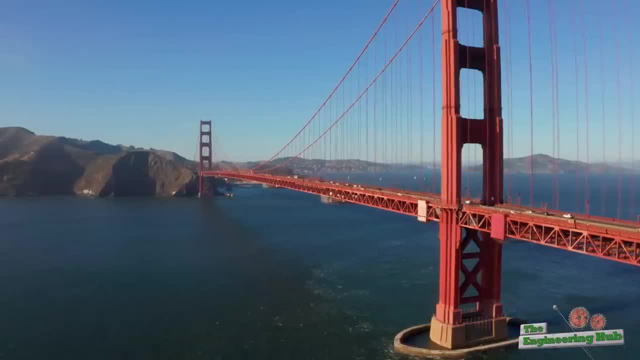 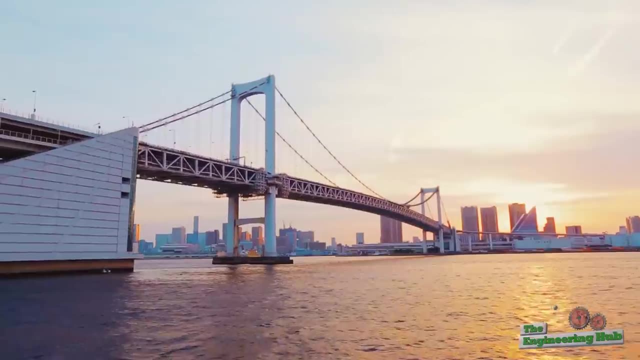 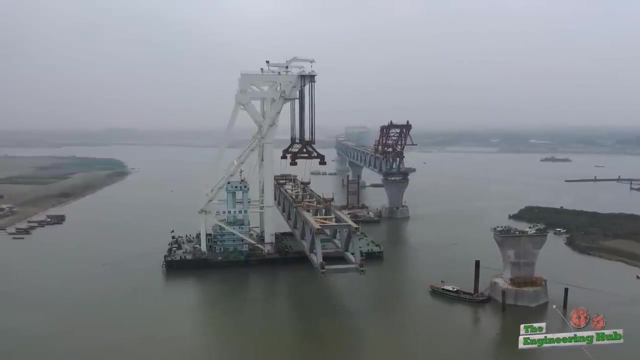 high flexibility very rarely have railway traffic unless the deck is stiffened with a truss-like structure. Let me know in the comments if you know of any purely suspension bridges open to railway traffic or any cool bridges in general. Trusses do also have disadvantages, for example buckling of. 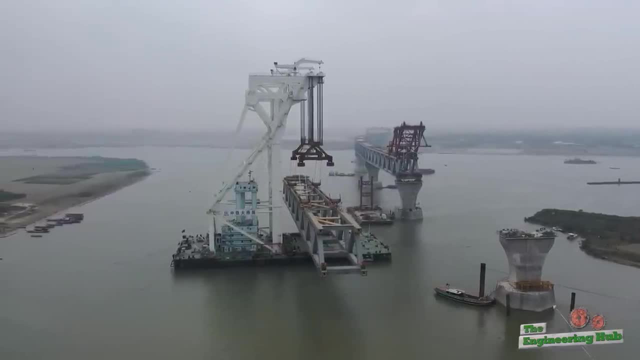 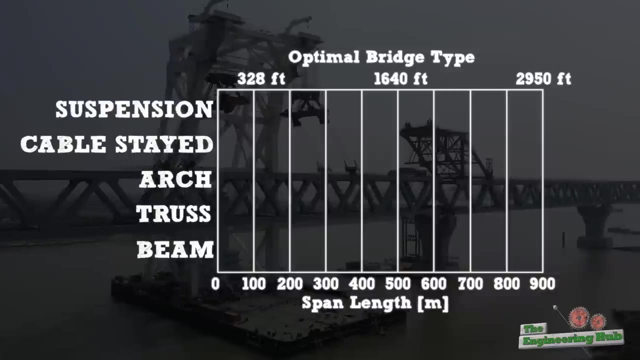 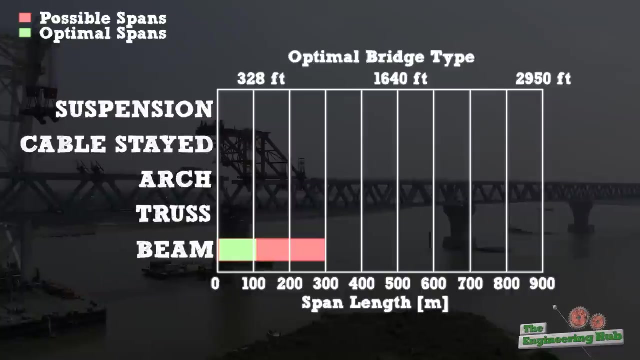 the compression element, increased construction complexity, and so on. Depending on the length, the effects of these parameters determine the feasibility of a particular bridge type. Beam bridges, due to their low material utilization but ease of construction, are the preferred choice for spans of up to 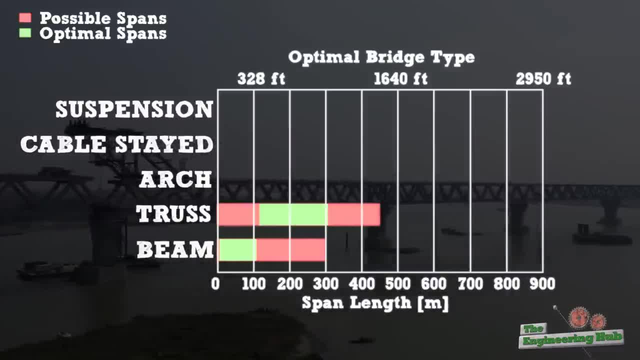 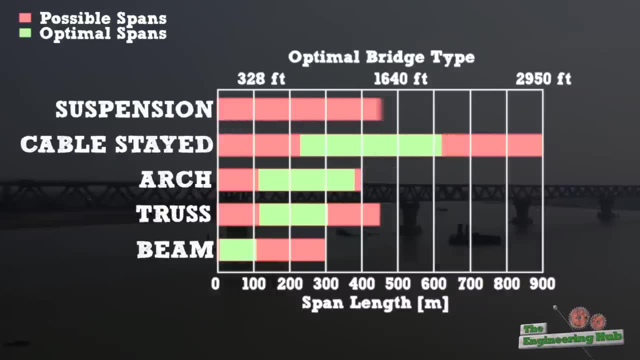 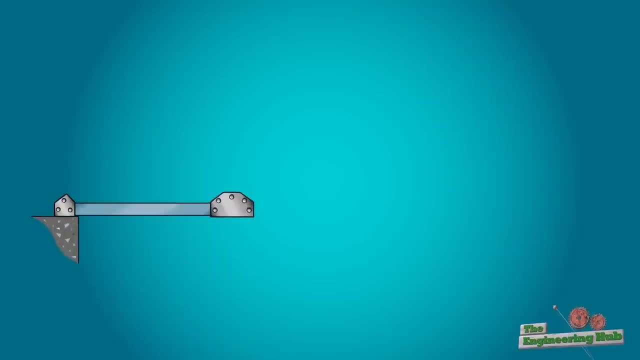 100 meters, Beyond 100 meters and up to 300 meters, the truss becomes the optimal bridge choice. For even longer spans, the cable state and suspension bridges become optimal. In many cases, a combination of these techniques is used. The truss is efficient because its members. 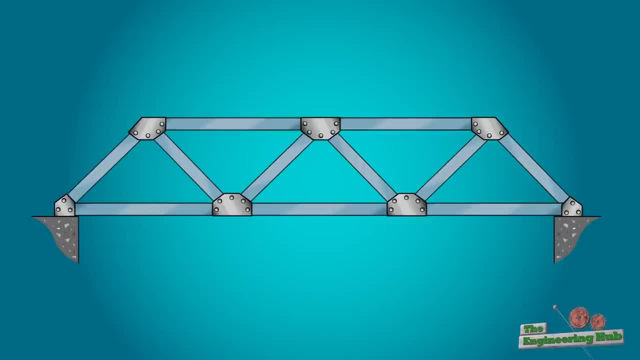 do not need to be fixed, But it feels like we still haven't explained why this is the case. Why do truss elements not bend? Our intuition suggests otherwise. When elements are loaded perpendicularly, they should be bending. In the case of the, 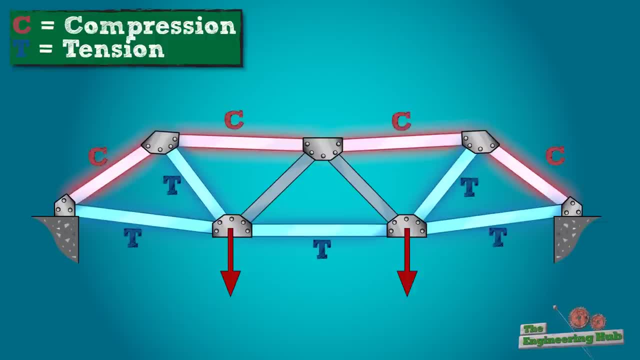 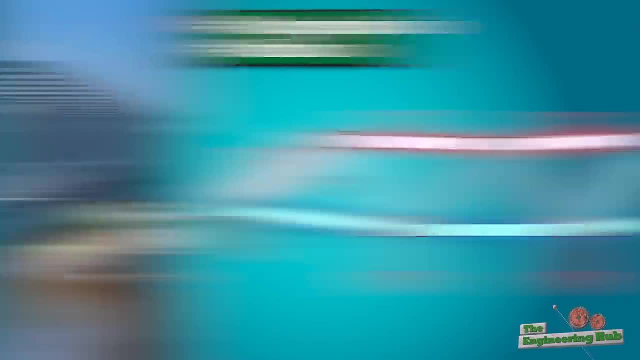 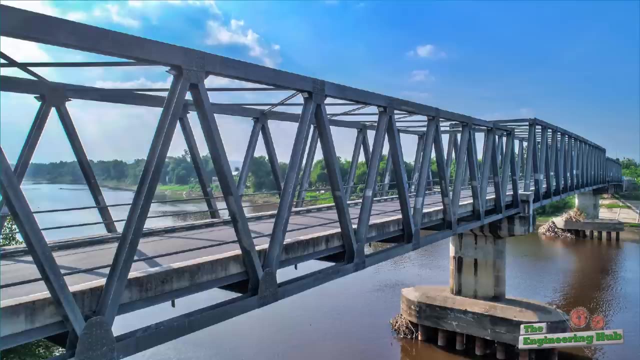 truss. the overall structure is bending, but its individual elements are not. They're only being compressed and stretched. There are two main reasons why this is the case. The first reason is because trusses are usually only loaded at the joints. This is not always obvious, but if you have a closer look at a truss assembly you can. 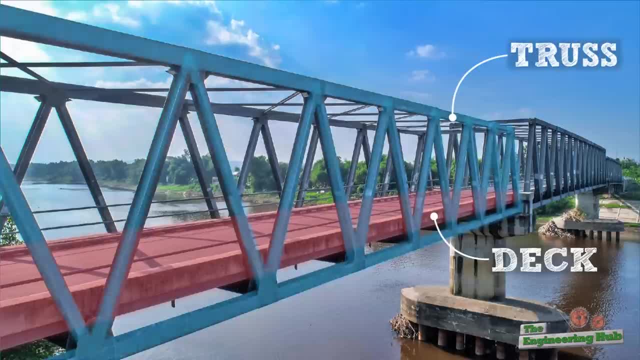 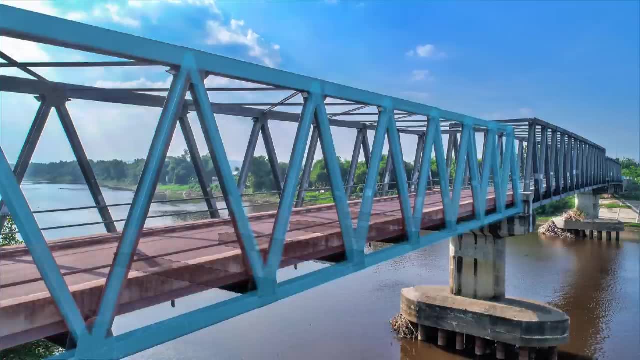 see that the deck is usually not directly attached to the truss itself, but it's resting on floor beams that run in a perpendicular direction. The floor beams are then connected to the joints, where the load is distributed into the truss and then transferred to the 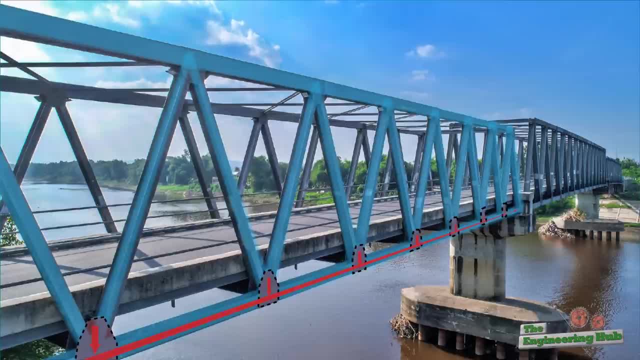 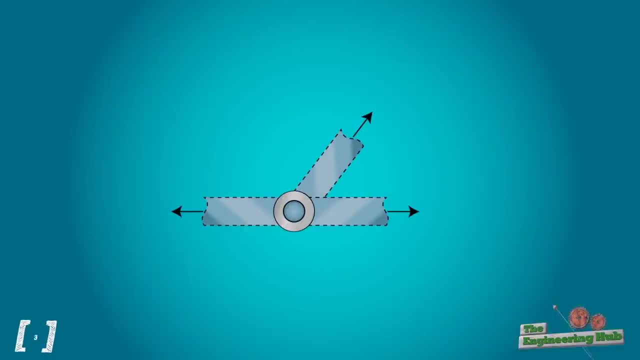 end supports. The second reason is less obvious and requires a slight understanding of statics In engineering. the joints of a truss are modeled as pin connections, which means the members can freely rotate around the pin, But in reality, we never see these pins. in fact, we see heavy gusset plates. 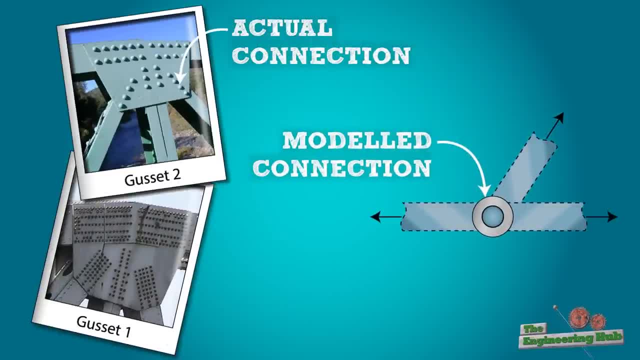 scattered with dozens of bolts. Surely this cannot be a pin. Well, it's not an actual pin, but the connection does behave like a pin as long as a very important condition is satisfied: The requirement for the gusset connection to behave as a pin. 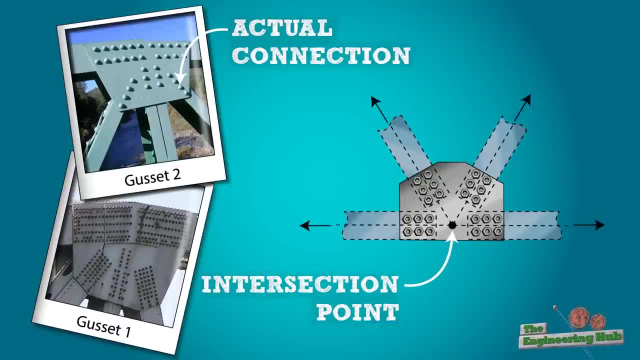 is that all of the connected members intersect at the same point. If they do, then there are no couple moments generated at the joint. In contrast, if one of the members was installed incorrectly and did not intersect at the same point, then for the joint to be in equilibrium there has to be a bending moment present. 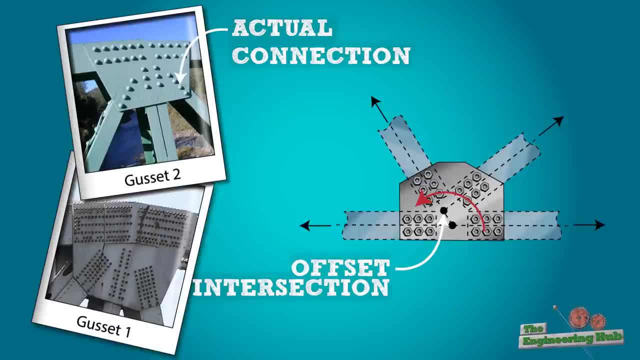 This becomes obvious if we sum moments about the intersection point, which clearly leads to a non-equilibrium condition which can only be balanced by bending of the offset member. Of course, in reality the connected members are not perfectly intersecting, but as long 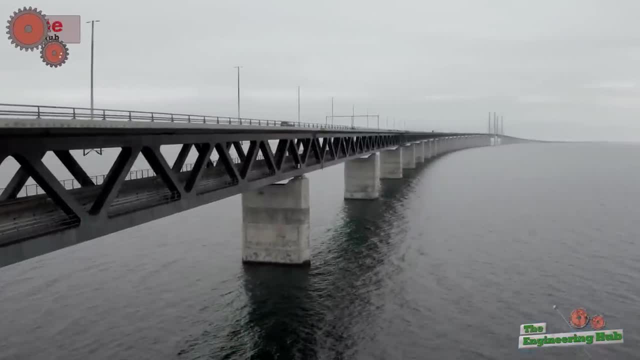 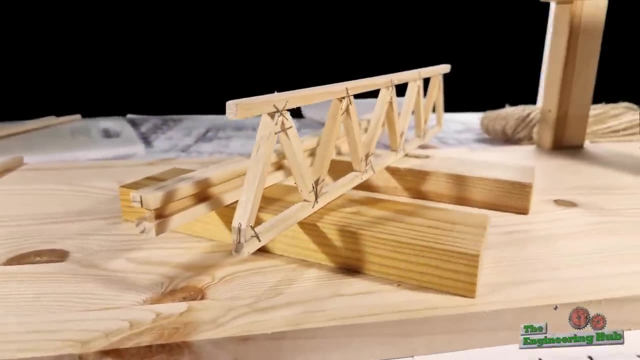 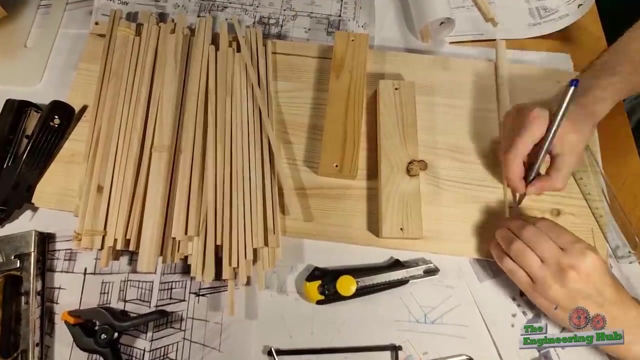 as they satisfy a particular tolerance, then the pin assumption holds and the structure is incredibly efficient. Now let's see a practical example of a Warren truss compared to a beam of the same cross-sectional area. I decided to go with a Warren truss mostly because, of course, of course, of course. 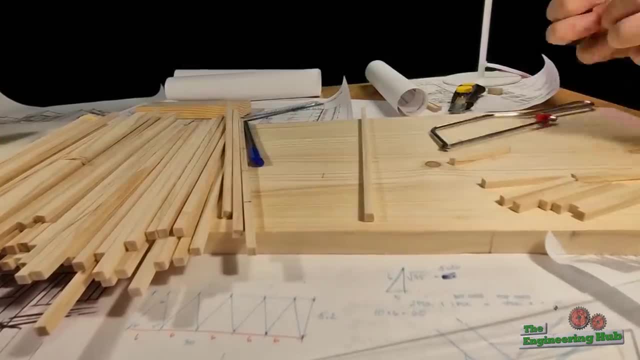 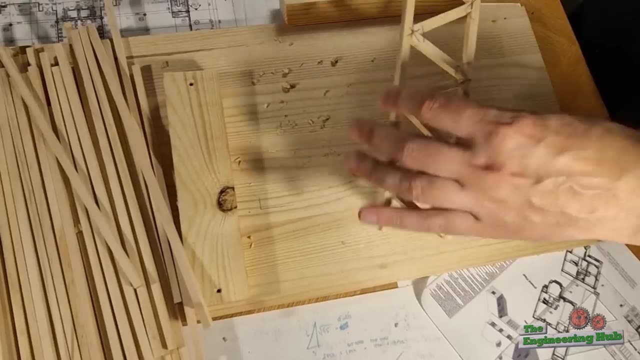 all members are of the same length, so it was supposed to be easier to cut and build. My craftsman skills are limited, so, as you can notice, the truss is far from perfect. The beam was significantly easier to build, since it was only about gluing the sticks. 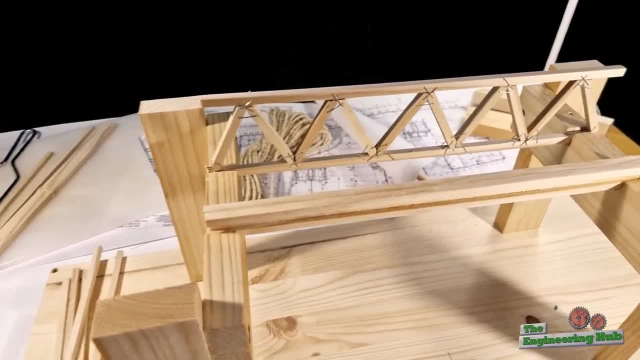 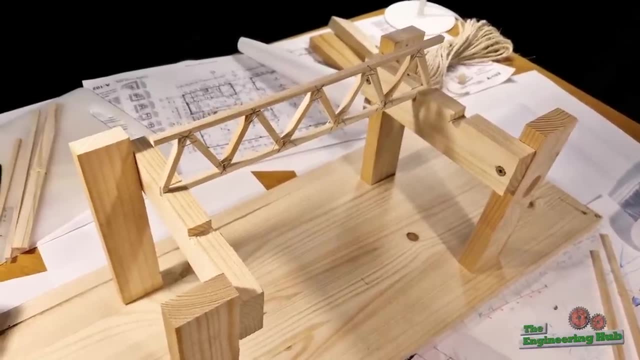 together. Even though these are far from real bridges, they do to some extent reflect on the difference of man-hours required for each structure. For that reason, the beam bridge is sometimes preferred. For that reason, the beam bridge is sometimes preferred. 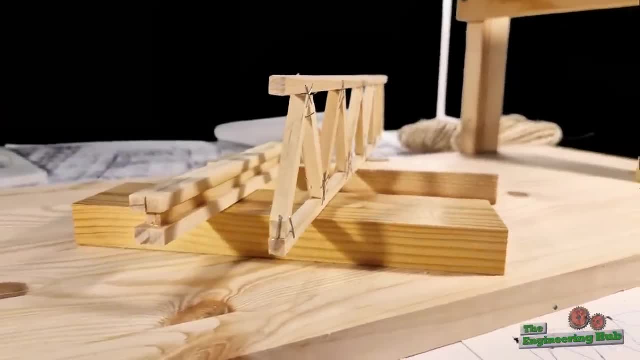 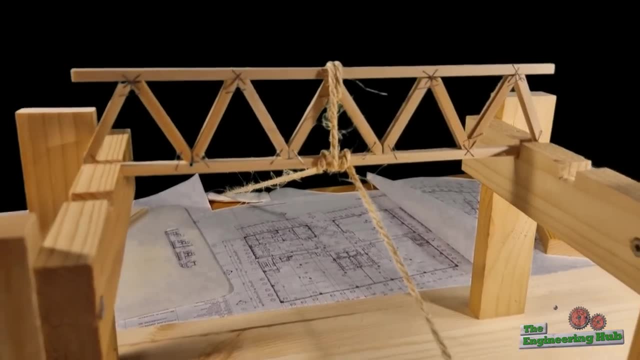 From a material point of view, the beam is less efficient, but the extra material expenses are quickly recovered due to the simpler construction. The loading was performed with a bucket of wet sand hanging under the table For gravity. only the final stage is shown here. 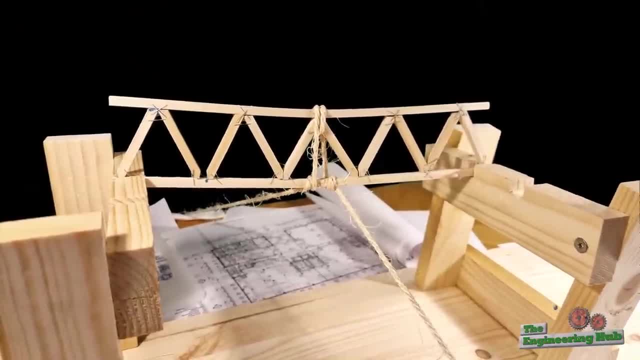 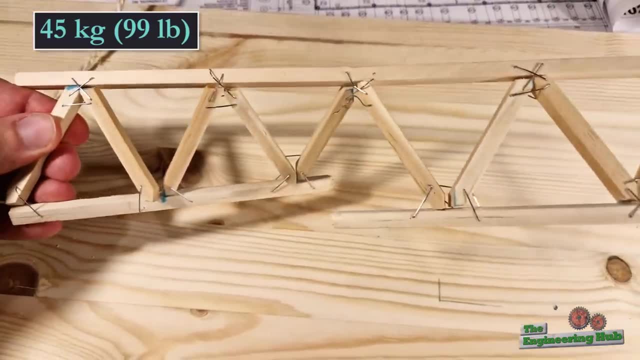 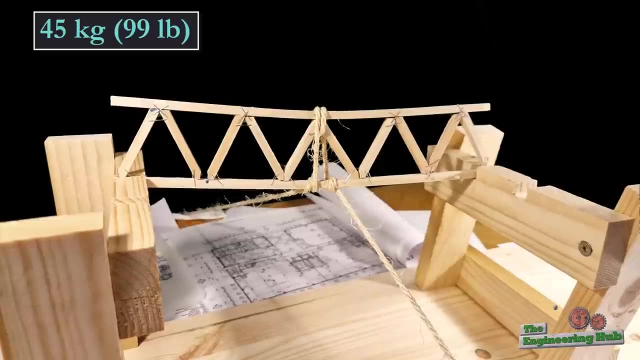 The truss managed to carry 45 kilos or 99 pounds before failing. In reality, a better constructed truss would have performed much better. Also, the failure was not pure luck. It was a failure. It had a significant amount of bending and sideway twisting which would not appear in. 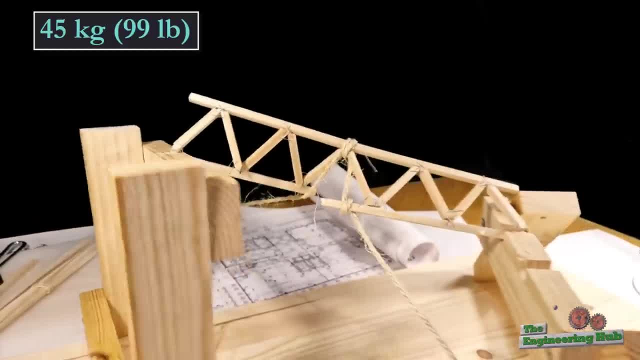 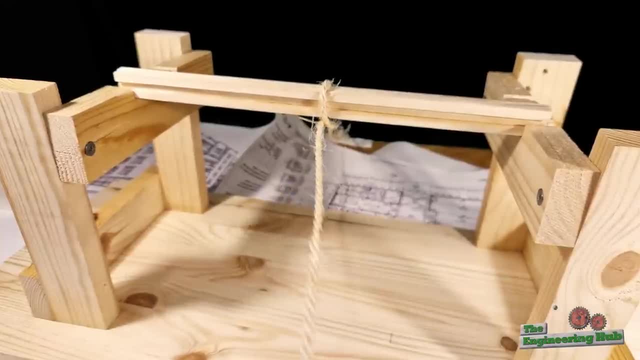 a real structure, as we discussed earlier. I know this experiment is far from perfect. I will try to get better in the future, so try not to be too harsh in the comments. The beam, on the other hand, performed fairly decent and reached 38 kilos, or 84 pounds. 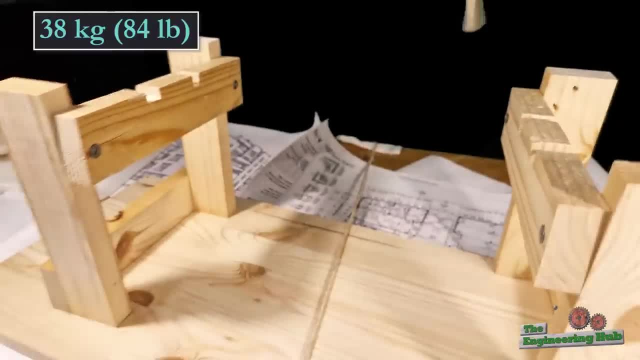 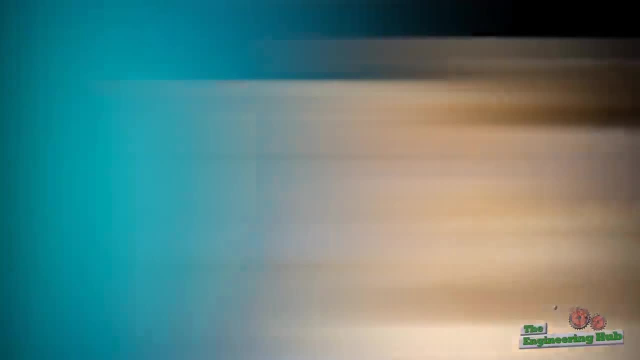 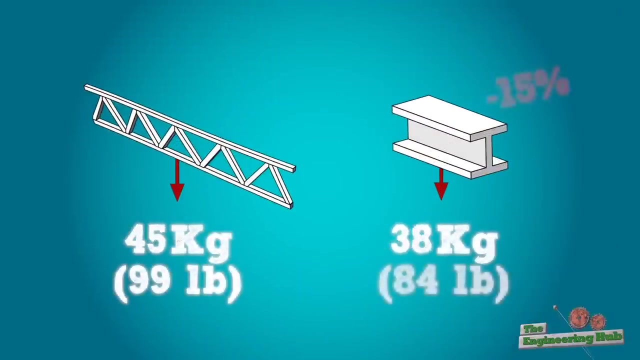 which is probably close to its real capacity, since it did not suffer from significant construction deficiencies. In summary, besides the poor construction, the truss still managed to outperform the beam by more than 15%, Depending on the application. this 15% difference, or possibly more, might be the deciding parameter. 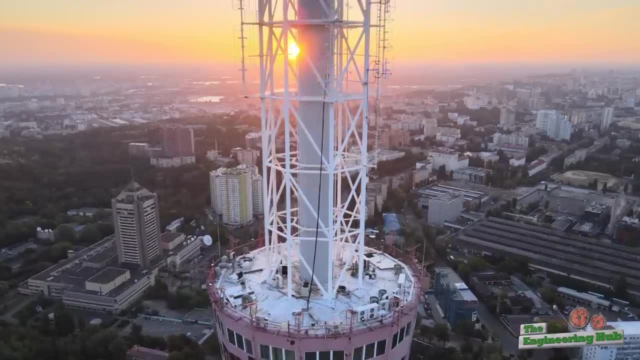 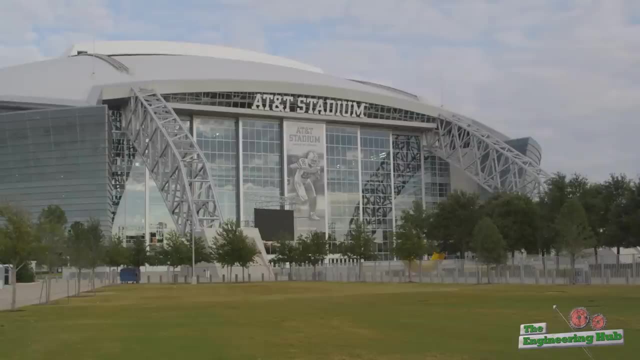 for going with a truss rather than a beam bridge. But truss structures do not appear only in bridges. You can find them in roofs, large venues, antennas and many other places. This video is a good introduction, But if you want to take your understanding to the next level, please subscribe to my 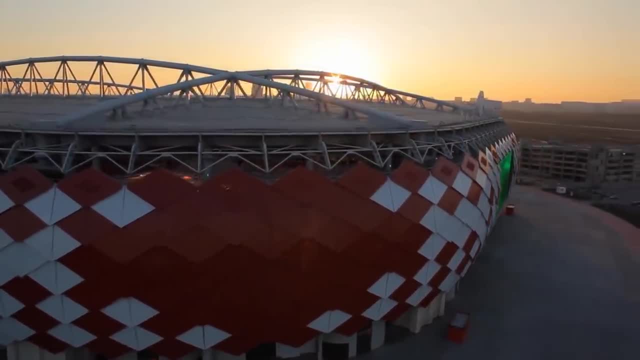 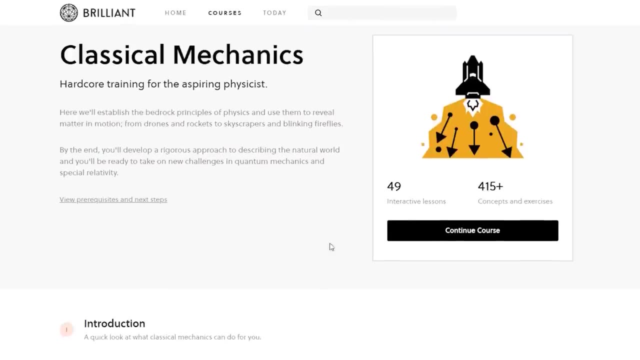 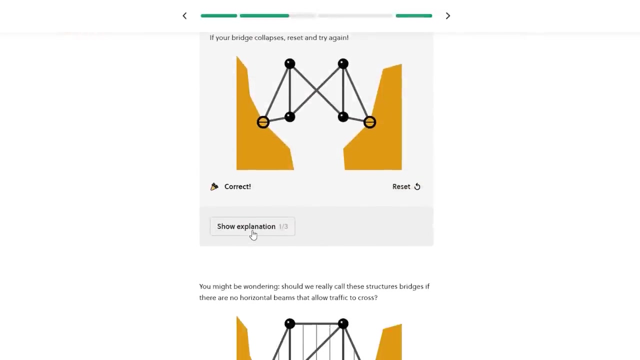 channel, You can check out the courses provided by today's sponsor, Brilliant. Brilliant is an interactive learning platform that helps you grasp complicated STEM topics through intuitive explanations and hands-on lessons. Brilliant has lessons on Newton's laws, statics, kinematics, even a specific lesson on truss. 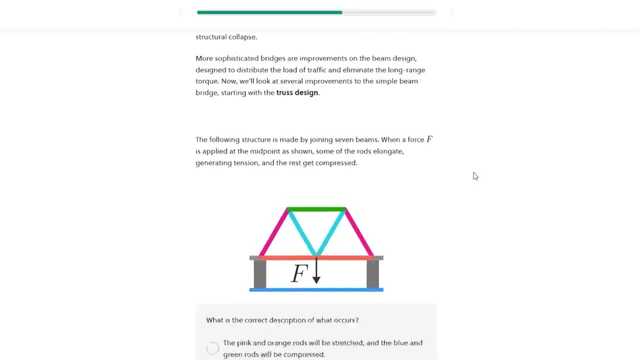 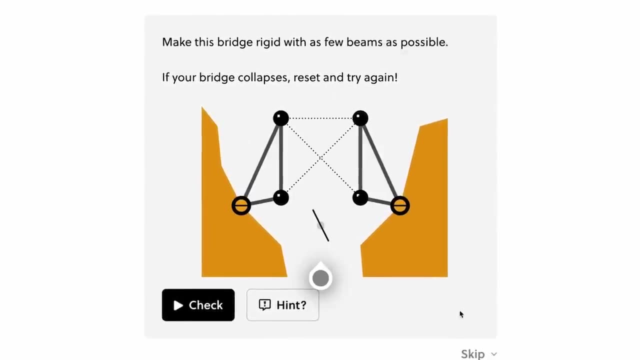 and beam bridges that explain in a bit more detail the theory behind these structures. The best thing is that the interactive visuals and intuitive explanations are so natural and entertaining that it could take you a long time to get used to them. Thank you for watching. 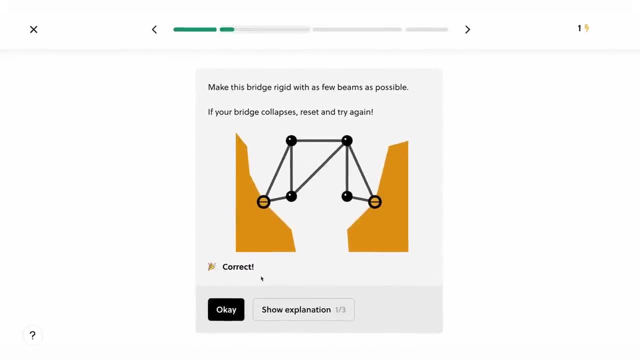 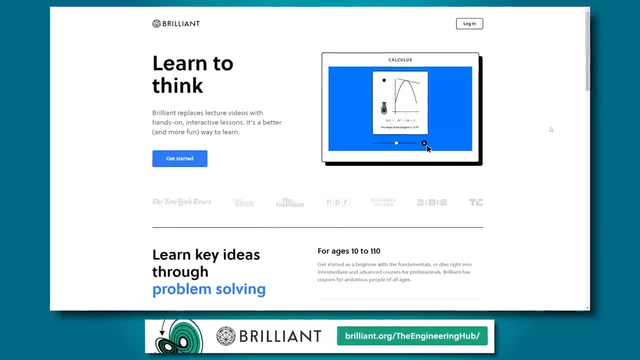 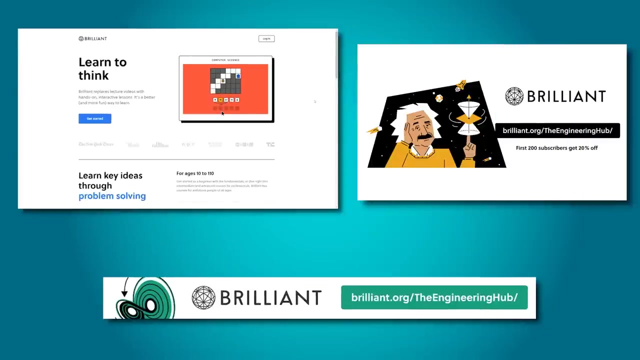 See you next time, Bye, bye. Brilliant is a program that completely takes away the feeling of a boring lecture room while achieving deep conceptual understanding. Head to brilliantorg forward. slash The Engineering Hub to get started for free with Brilliant's interactive lessons. The first 200 viewers will also get 20% off on an annual membership. 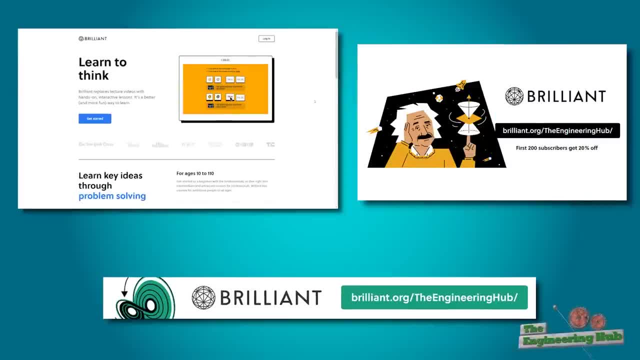 You can find the link down in the description. Thanks for watching. If you liked the video, consider giving us a thumbs up and also subscribing to our channel. Thanks for watching. If you liked the video, consider giving us a thumbs up and also subscribing to our channel.